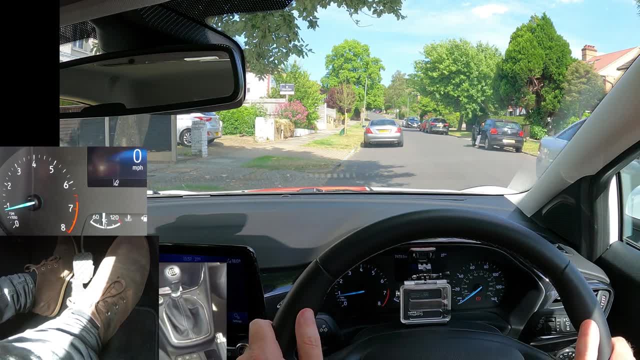 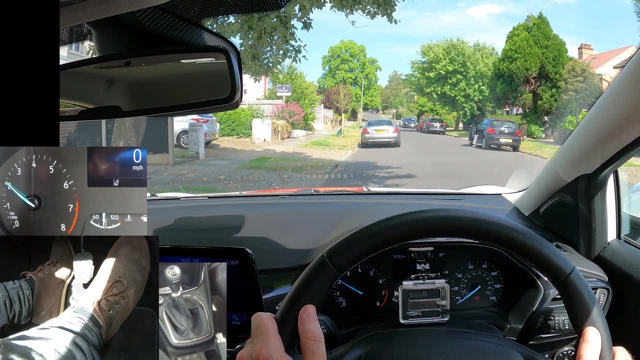 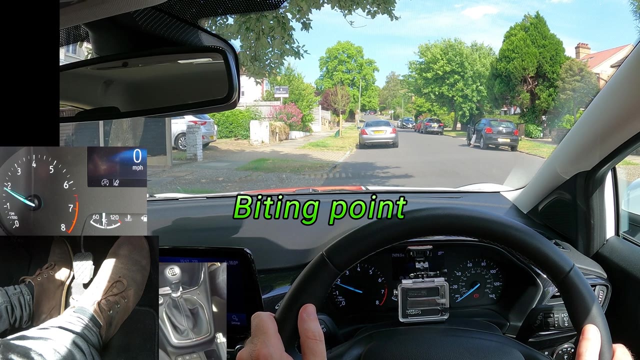 need to get it relatively quickly. You know when you've got a biting point, as the back of the car will dip down and the front will raise slightly To help prevent stalling. always set the gas before getting a biting point. On an uphill start, try and keep the revs a little above one and a half. 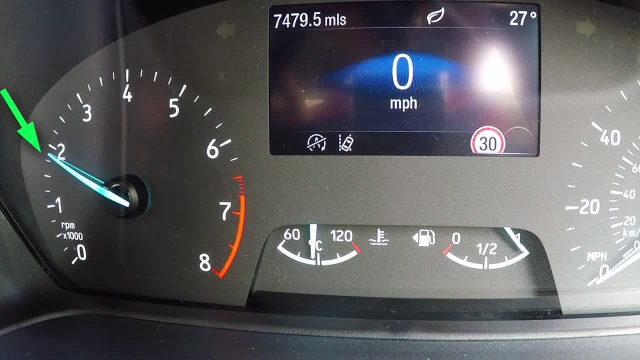 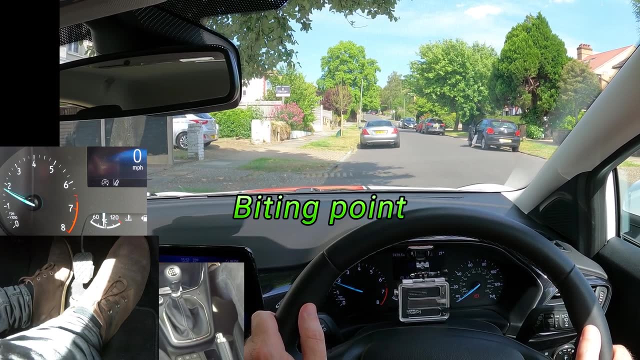 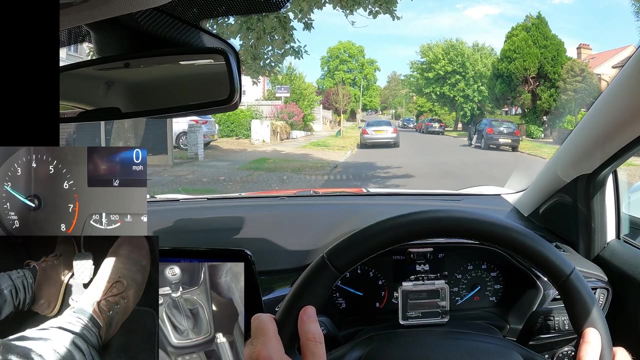 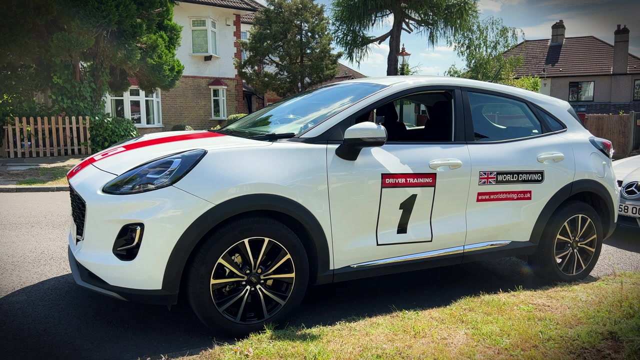 but it's not precise. If you don't get the biting point when doing a hill start, then the car will roll back, but if you raise the clutch too much, then the car will either stall or zoom off. This Ford Puma that I'm driving has hill start assist and it won't allow me to turn it off When 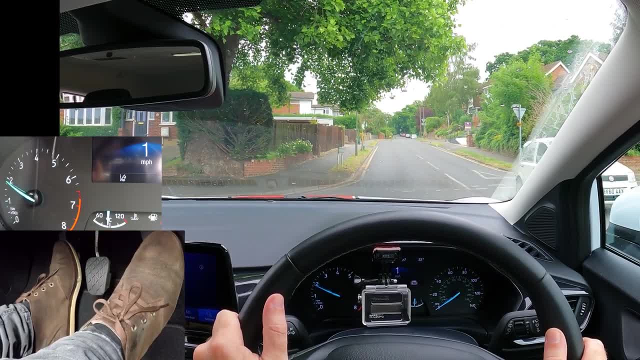 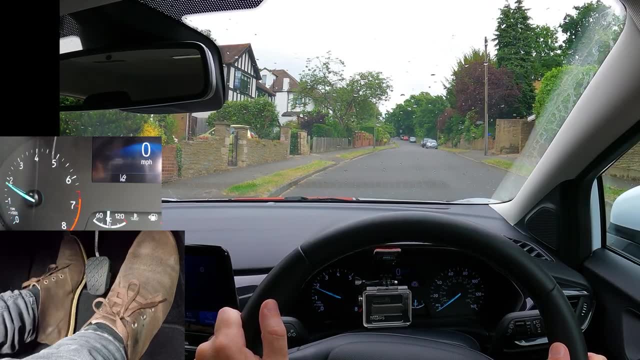 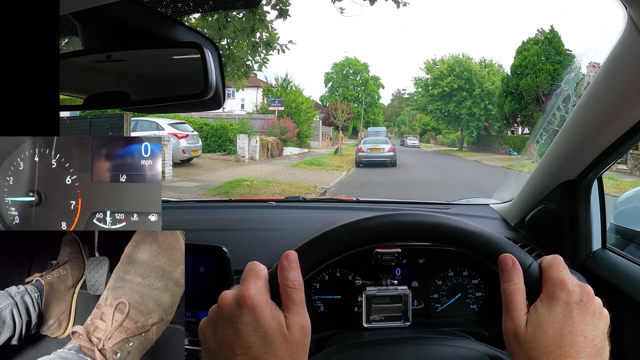 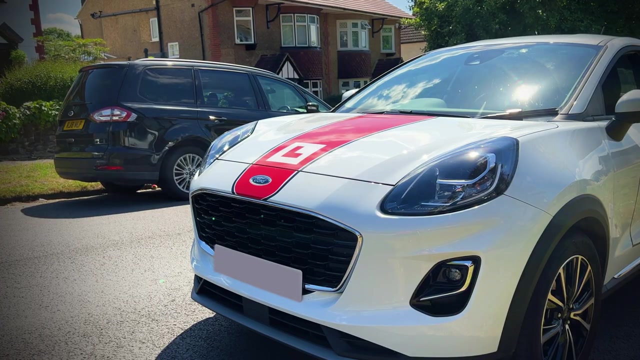 you stop on an uphill and release the foot brake, the car stops you rolling back for about three seconds. This is meant to give you time to get the gas and biting point, but take any longer and you'll still roll back. But as your car might not have this feature, I'm still not going to use hill start assist. 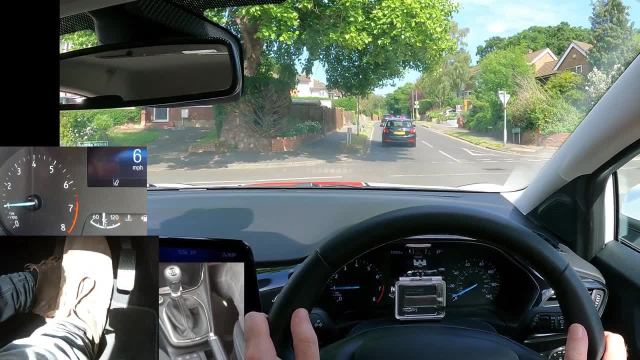 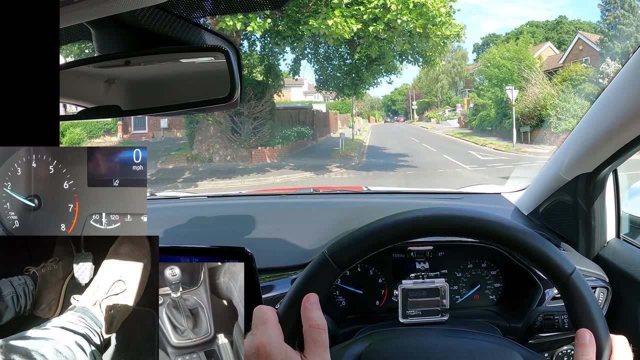 The first technique I'm going to show you involves the parking brake. You might think that it's a big hassle and takes ages to apply the parking brake like this and release it, And for some new drivers it can take a minute. But let me show. 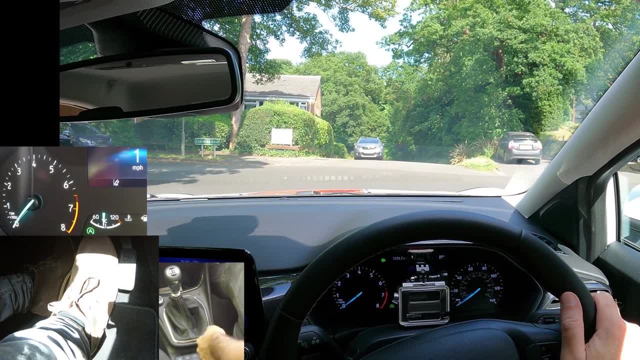 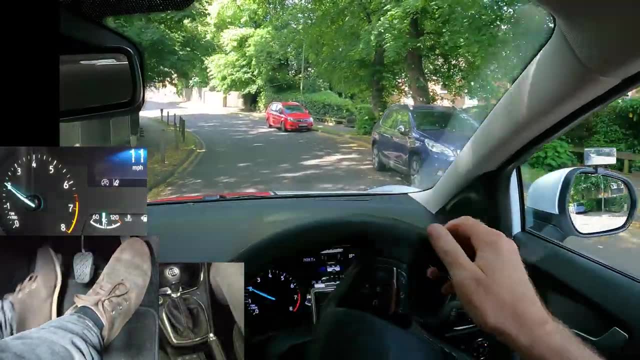 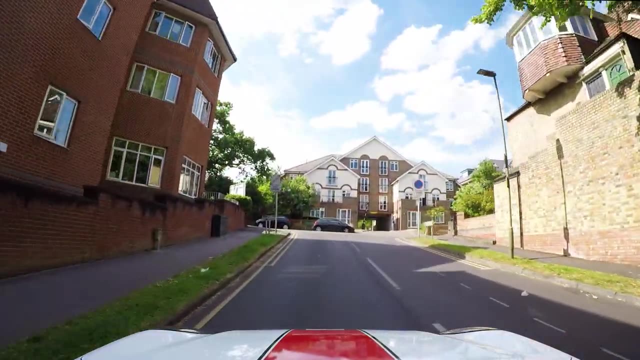 you how quick you can apply the parking brake, prepare to go, release the parking brake and make hill starts really easy. All of the junctions I'm going to show you today have give way lines and I don't have to stop completely as long as it's definitely clear and safe. but I will be stopping to. 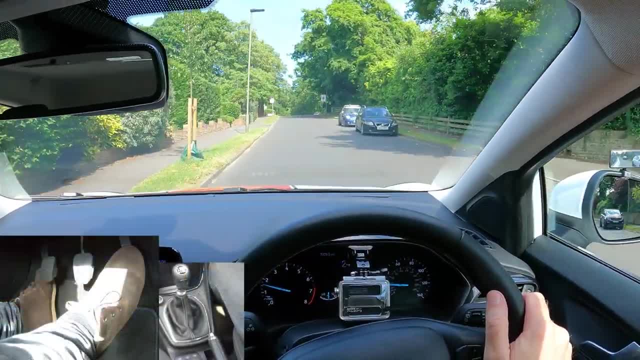 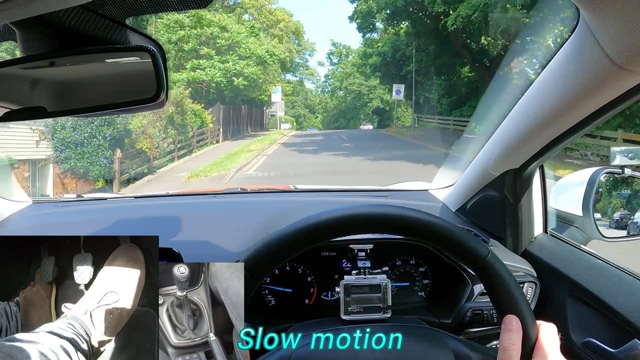 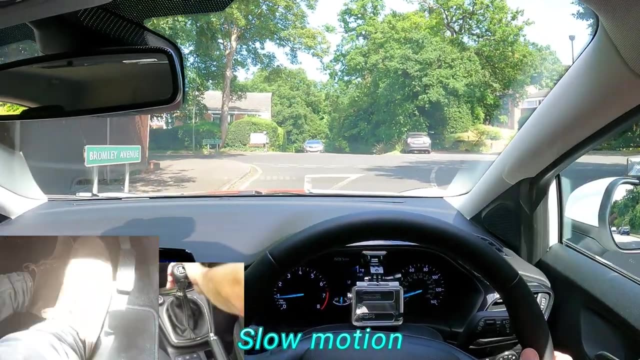 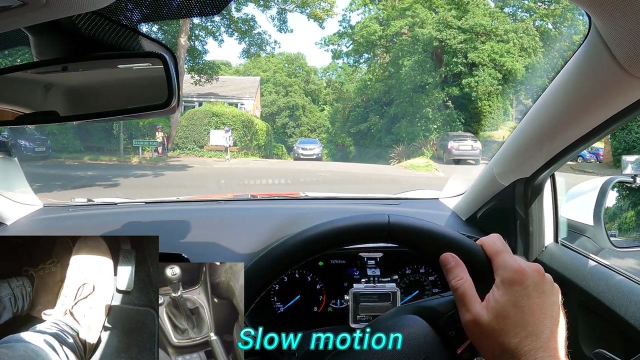 show you some hill starts. I'm going to show this first junction in slow motion. As you approach the stop off gas Brake lightly, as the hill will slow you down quite a bit quickly. Clutch down first gear Once you've stopped parking. brake on if you're only here. 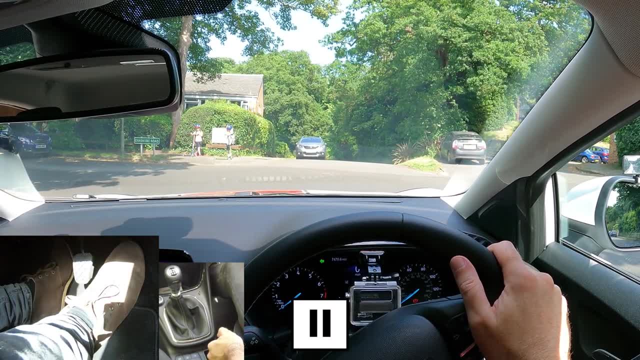 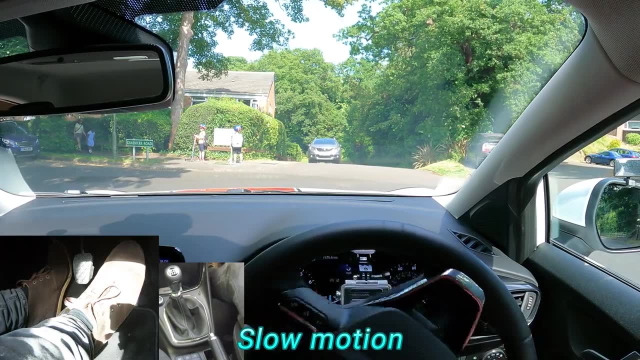 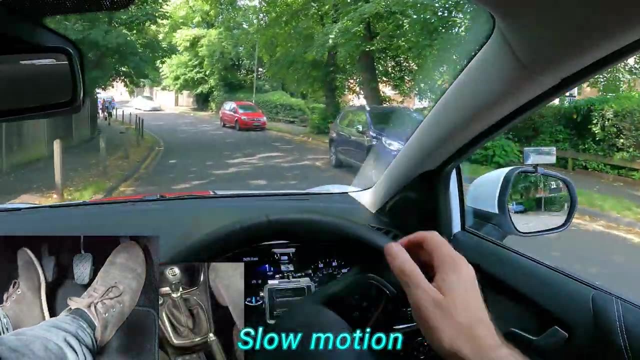 for a second and leave your hand on it to save time. Make sure it's safe gas biting point: release the parking brake a little more gas as you keep the clutch steady. Then slowly release the clutch with more gas. Here's the junction: again at normal speed. The benefit: 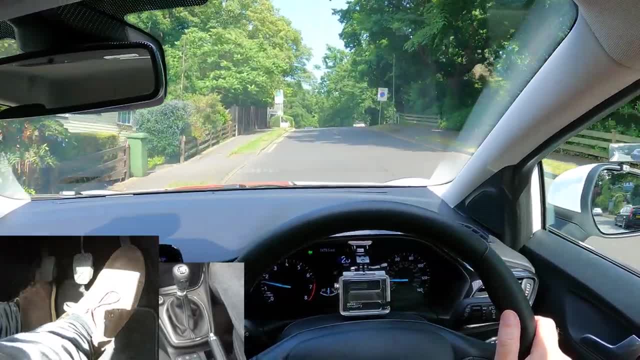 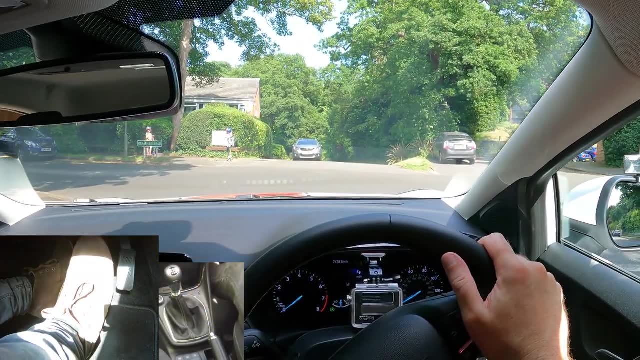 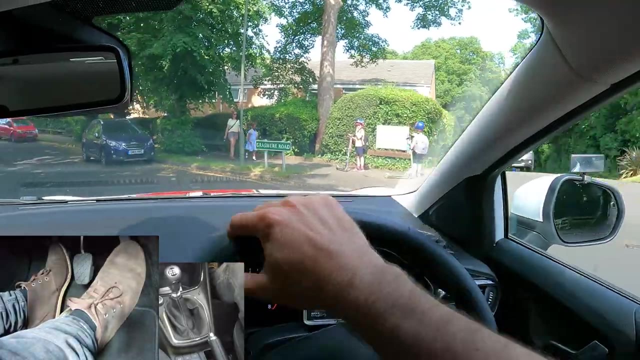 of using the parking brake is that it allows you to prepare the car to go again. Brake lightly as the hill slows you down. Clutch first gear Steer left slightly parking brake gas biting point: safe to go. release parking brake a little more gas clutch steady, gently. 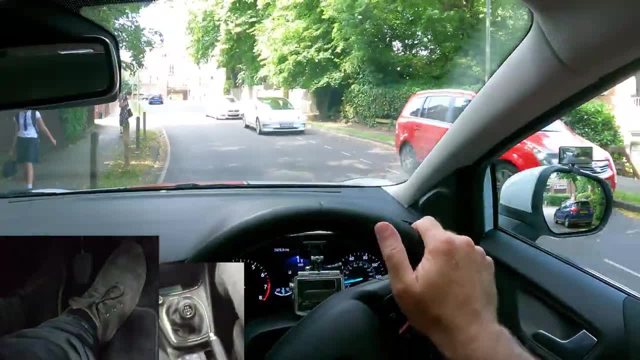 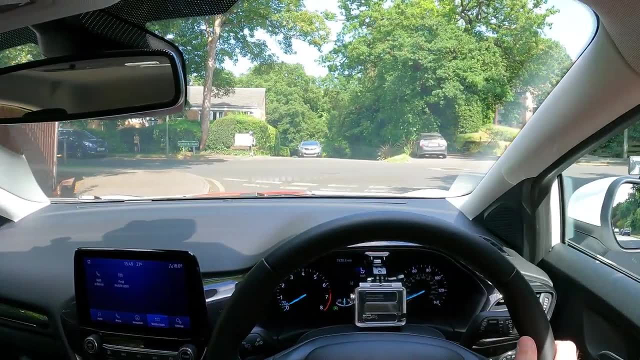 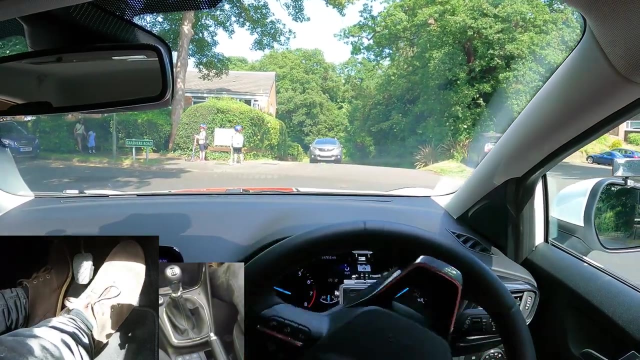 raise the clutch with more gas. It all happens so fast And it does take a bit of practice. Remember to lower the clutch slightly about the thickness of a pound coin if you're merging out of the junction a little quick, Or raise it slightly. 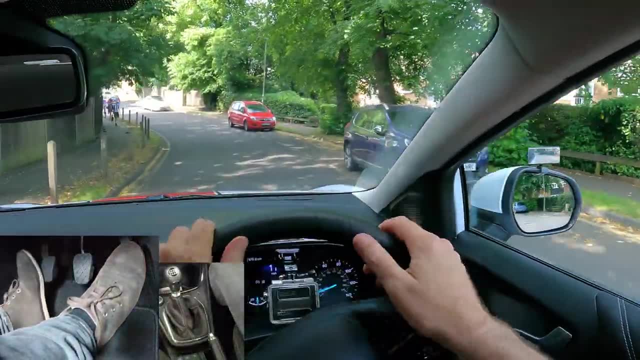 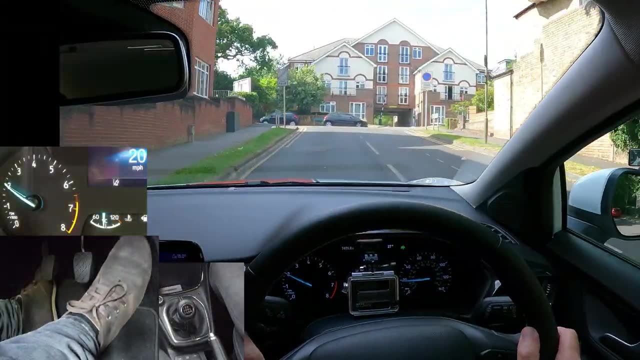 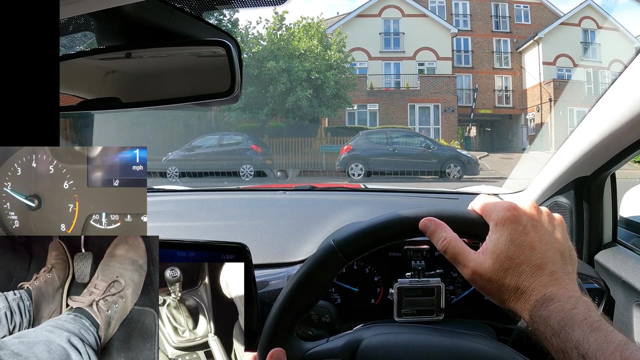 to increase speed. The hill will slow the car down. but if you feel like you're stopping too early, release the foot brake. then set the gas and biting point to creep forward. Don't forget to avoid stalling. always press the gas before biting point And don't release. 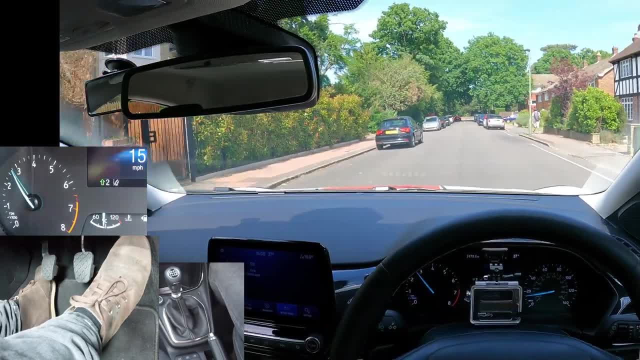 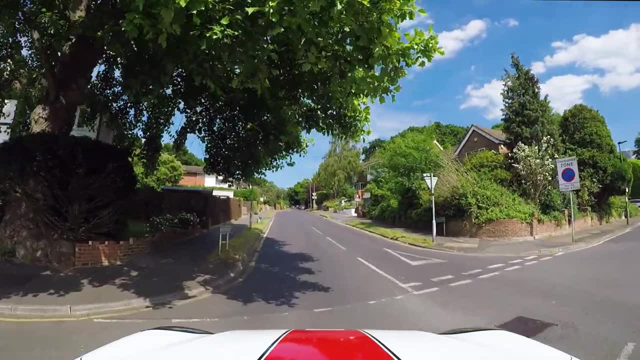 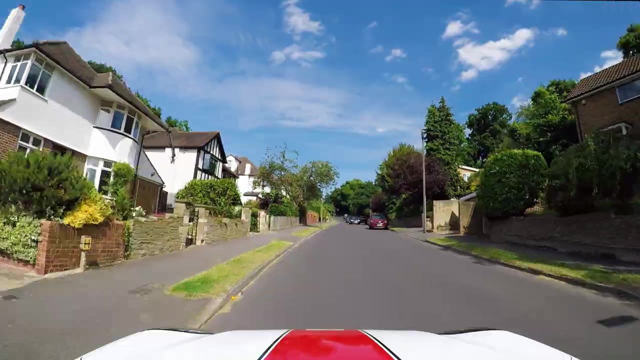 the clutch too soon. Hold on to it for about 3 seconds as you move off. When you do a hill start, try not to think about rolling back or stalling, Otherwise you'll be distracted and it might not work out well. My favourite way of dealing with a junction on a hill is…. 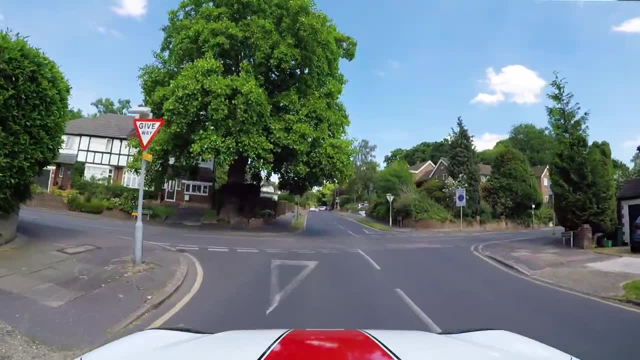 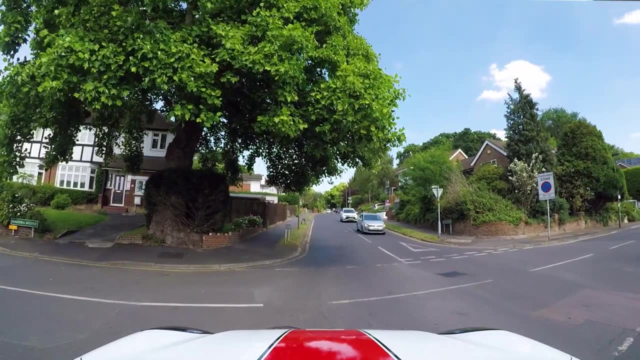 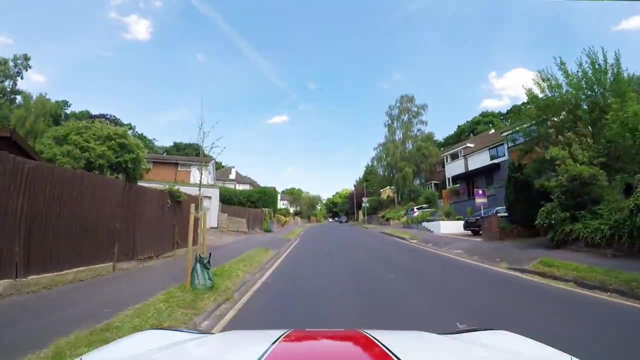 Well, try not to do a hill start in the first place, Instead not coming to a complete stop unless I had to Then using clutch control to creep really slowly. This does take a bit of clutch control practice, so let me show you. 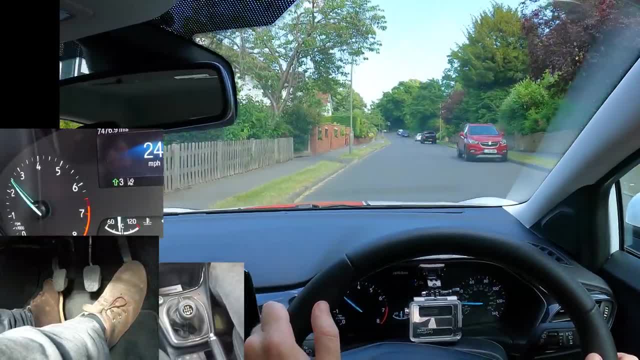 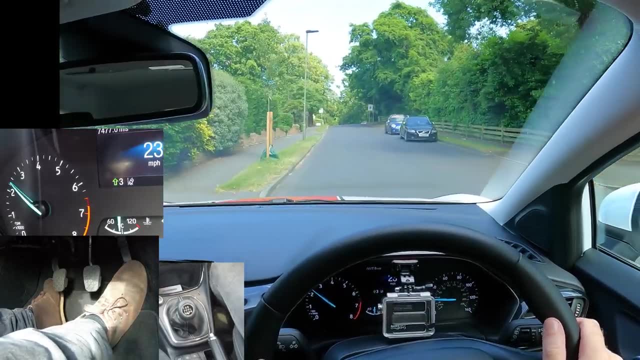 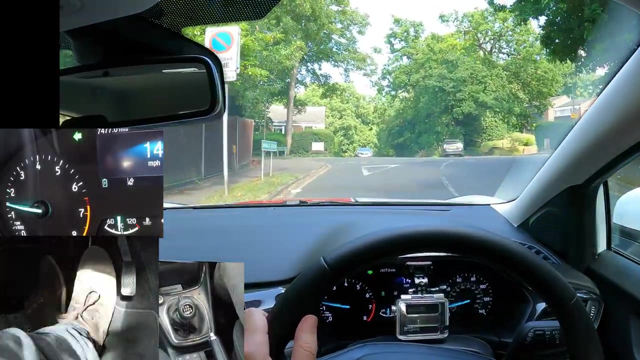 Approach the junction slowly, so you've got time to observe. Don't forget that the hill is slowing the car down, so you might not need to brake too much. Once the car has started to roll back, release the gas pedal, brake lightly, clutch down. 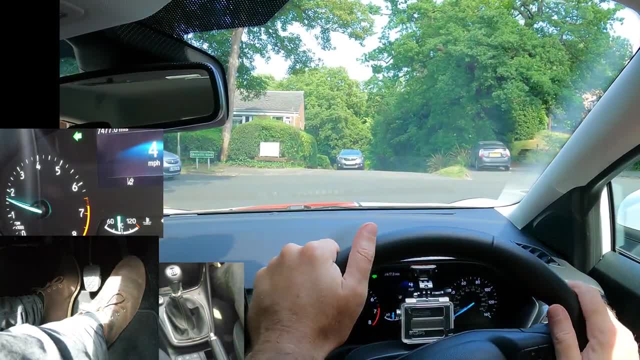 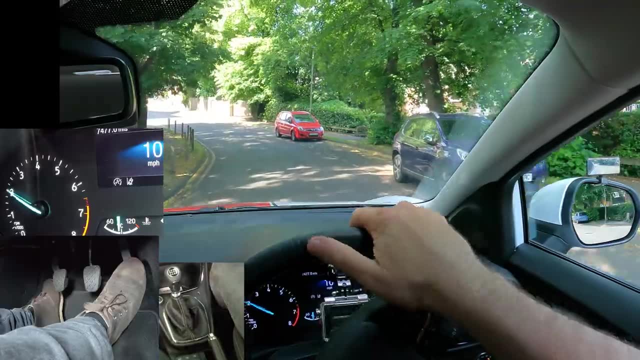 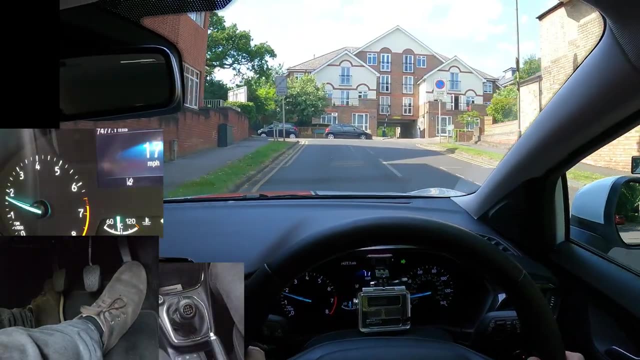 first gear. now gas and biting point to creep slowly. Observe lots for others and be ready to stop. Then gently raise the clutch with more gas to go Off gas lightly. brake clutch down first gear, Let's see what happens. Get into a corner and then head up to the left so you freeze. 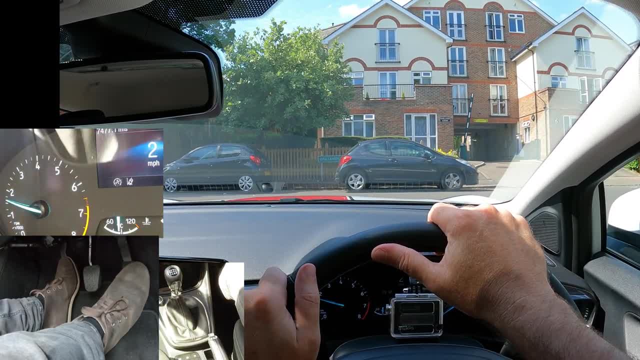 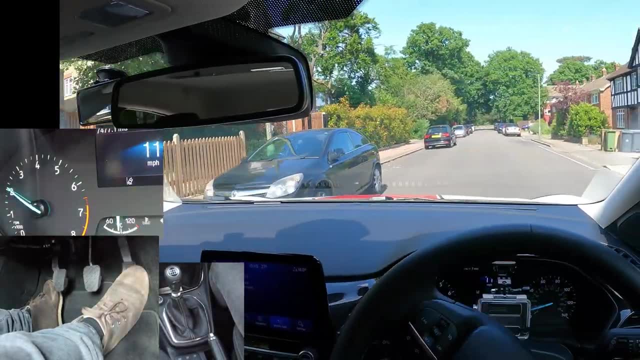 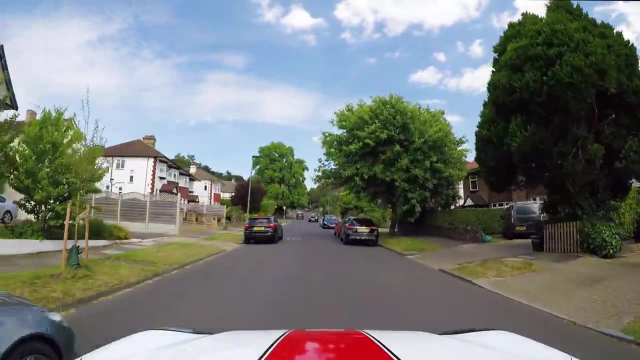 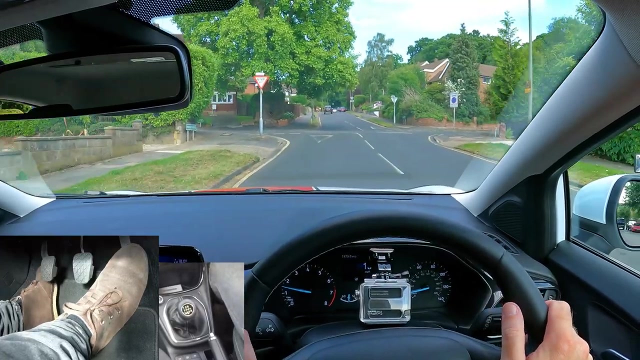 gear gas biting point. creep and observe loads, be ready to stop, then gas and gently raise the clutch. Don't forget that the hill is acting kind of as a brake. At the speed I'm driving I don't need to brake very much on the approach. First gear brake lightly. 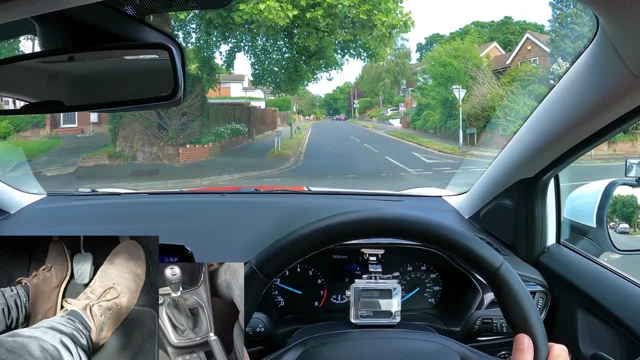 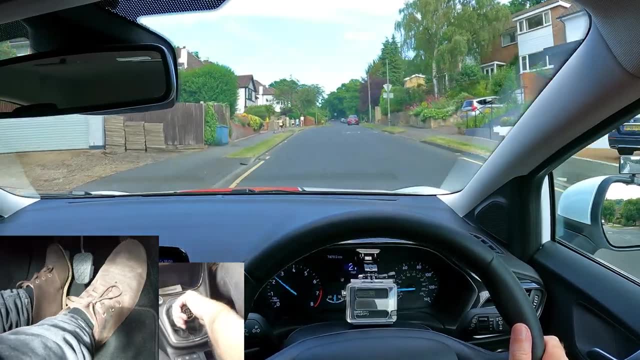 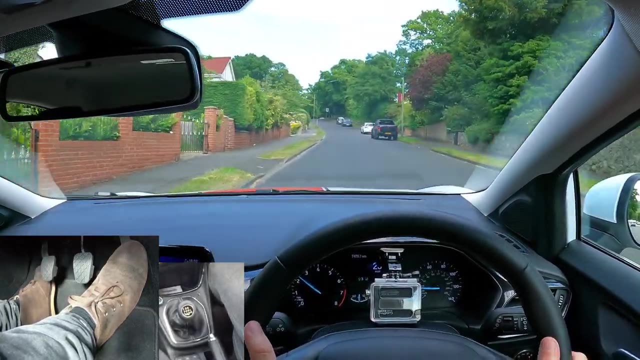 gas biting point. raise the clutch slightly to creep faster or lower it a little to slow down. Make sure you build up momentum before changing gear when driving uphill, as gravity will slow you down as you're changing gear. Otherwise you'll lose too much speed and the car will struggle. 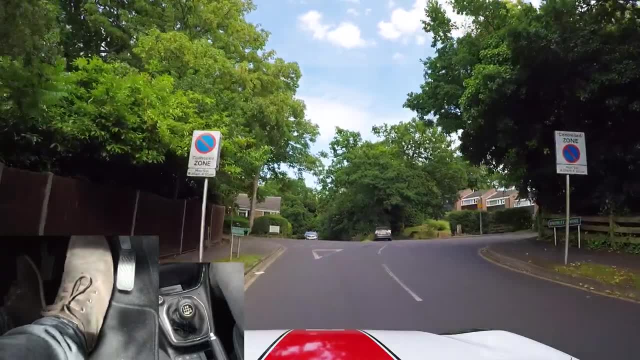 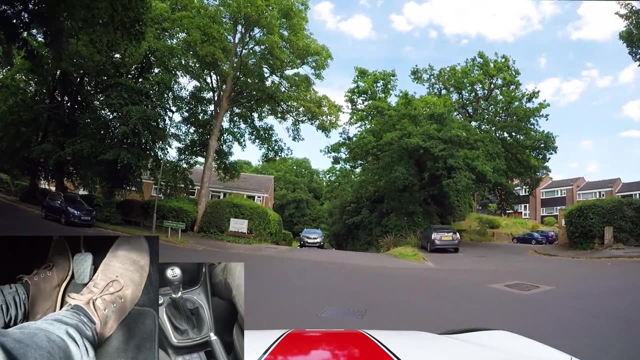 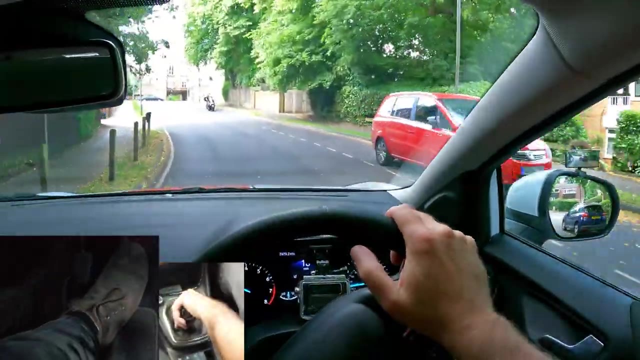 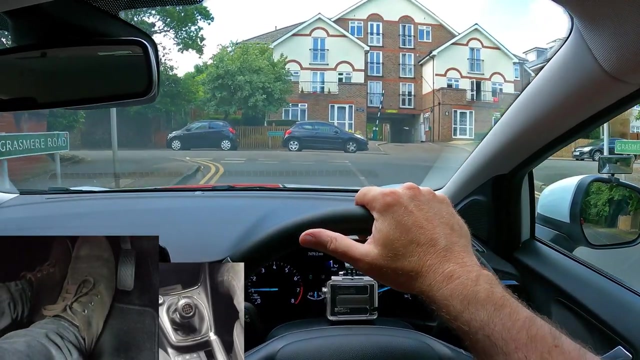 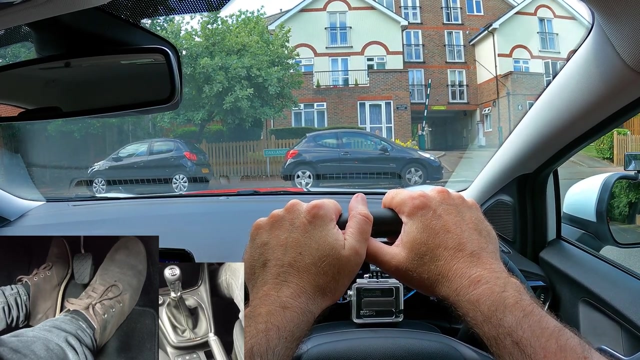 A lot of accidents happen at junctions, so always be careful, Always be ready to stop. Good, effective observations are so important. Gas, then biting point: Little movements with the clutch. lower it slightly to slow down, raise it a little to speed up, then gently release the clutch all the way. 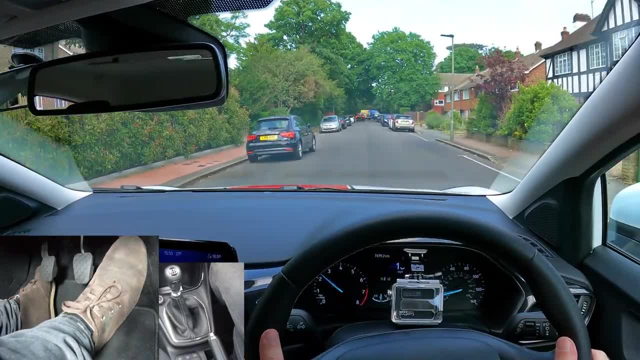 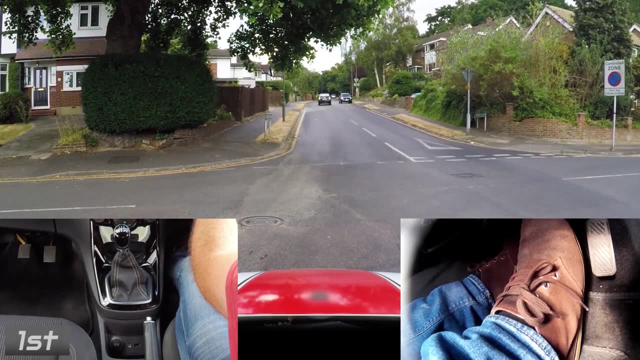 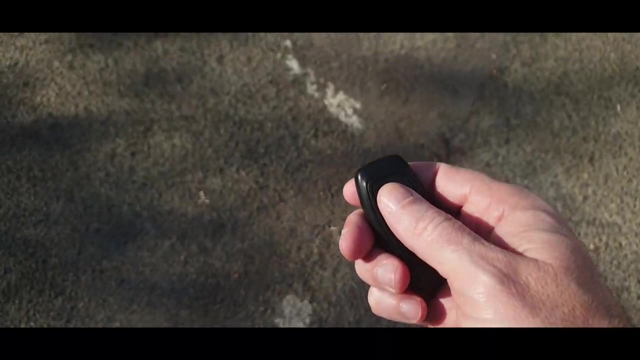 with gas to go faster. The other way to do a hill start is stopping and not using the parking brake. Instead, you'll have to be quick with your feet, setting the gas and biting point before the car rolls back. To do this, I'll have to. 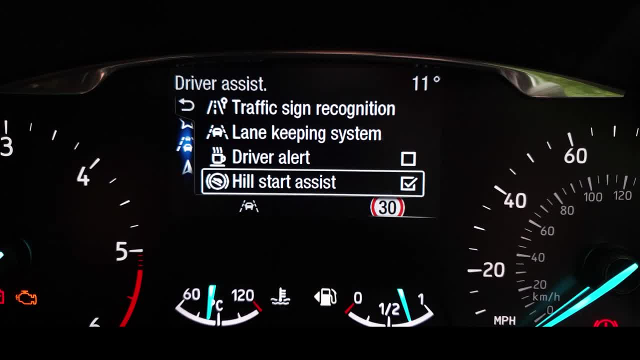 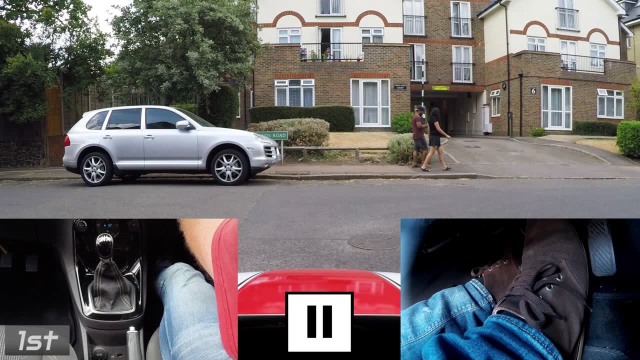 switch to a different car, as I'll be able to turn off hill start assist and show this way of doing a hill start. I've stopped at another junction. I'm going to be quick with the pedals Now. I could raise the clutch to the biting point with.